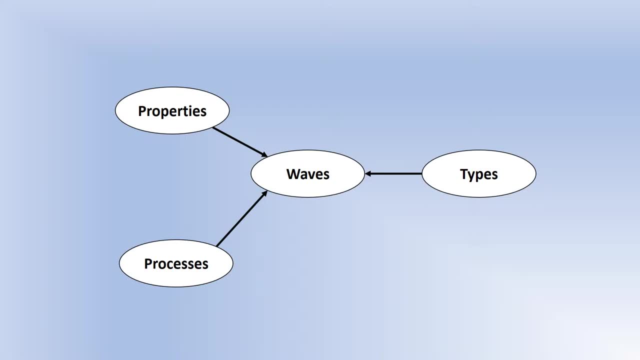 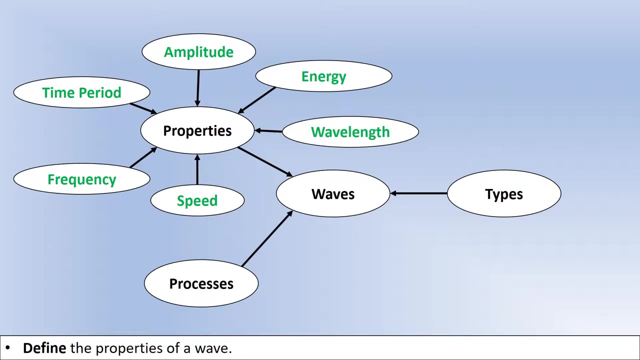 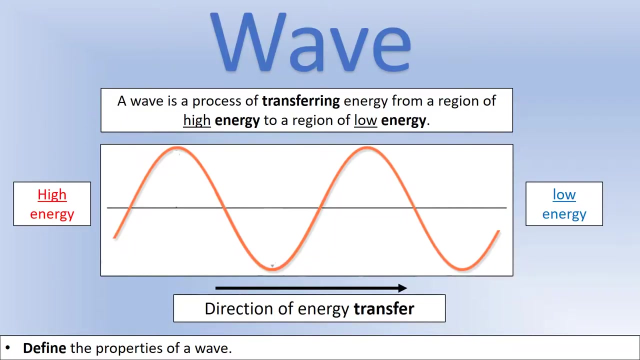 all of those other kind of processes that go with it. So we're going to start off looking at the properties, and there are six that we are going to focus on, and these are the things you can measure about a wave, and we'll explain what each of these six things are to start with. So let's first 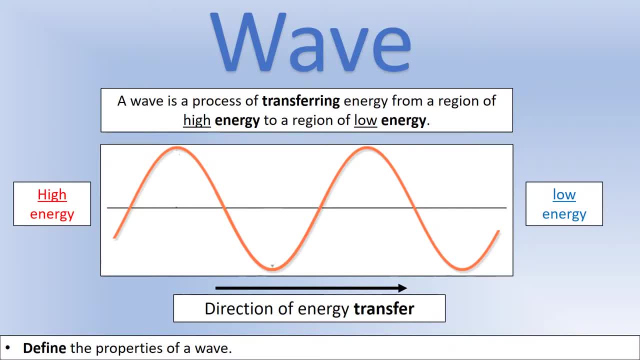 define what a wave is and link it in terms of energy. So you, a wave simply is a mechanism of moving energy from one place to another, and it will move it from a region of high energy to a region of low energy. so it might be something is very hot in. 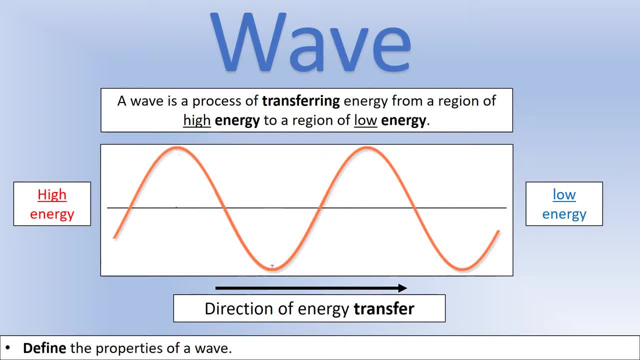 which case you get, like infrared radiation, moving energy. it might be that something just has a lot of potential energy and you just get a wave moving. there are lots of ways of doing it, but, simply put, a wave is a mechanism to move energy. okay, so let's move on to some of the things we can measure. 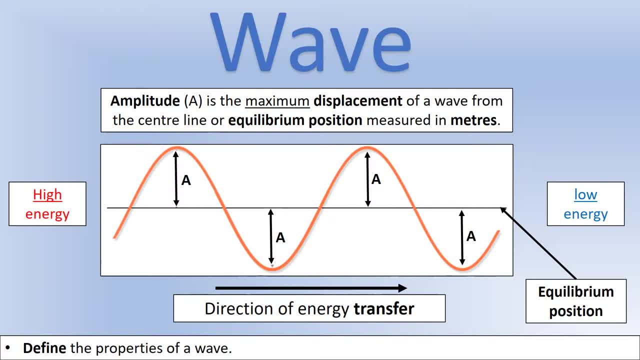 about a wave. so the first thing we are interested in measuring, because it tells us about the energy of the wave, is the amplitude which we give the symbol a, and this is an expression of the maximum displacement of a wave from the center line which we often call the equilibrium position. 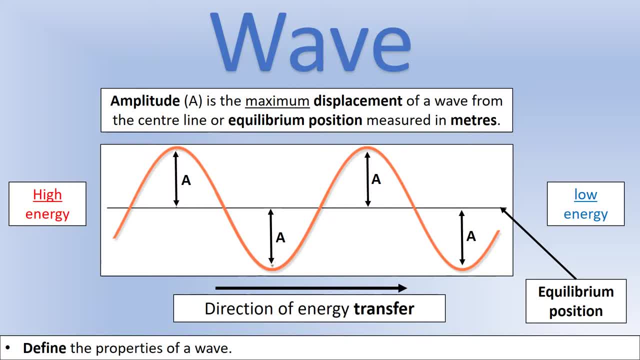 and that's the one you can see running through the middle here, and we measure the amplitude in meters, because it's a distance from this equilibrium position. okay, so that's the amplitude. the next thing we measure out a wave is the distance between peaks of the wave, and or we can measure it between any two identical points on the wave. it should come. 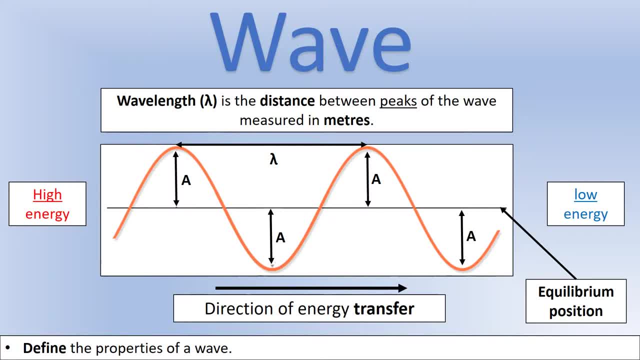 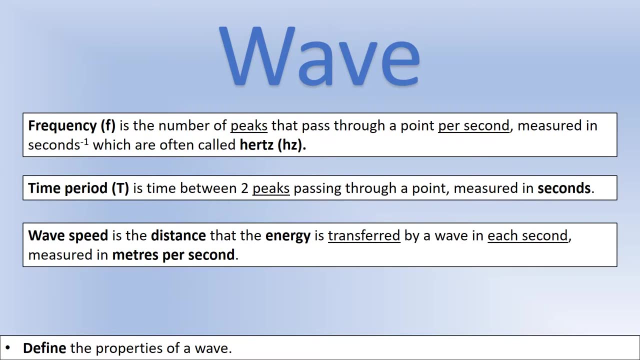 out as the same distance, but this is the easiest one to show. so this tells us how long one wave is, or one full wave cycle is. measure again, it's a distance and you can see it's shown on the diagram there. okay, so then there are a few other. 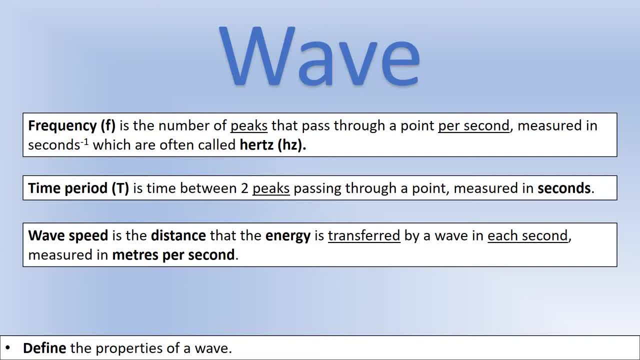 ones that we can measure as well, um, that are more tricky to show on a diagram. so the first is frequency, which is the number of peaks that pass through a point each second, or it could be the number of troughs that pass through each point second. it should be the same value, and that's. 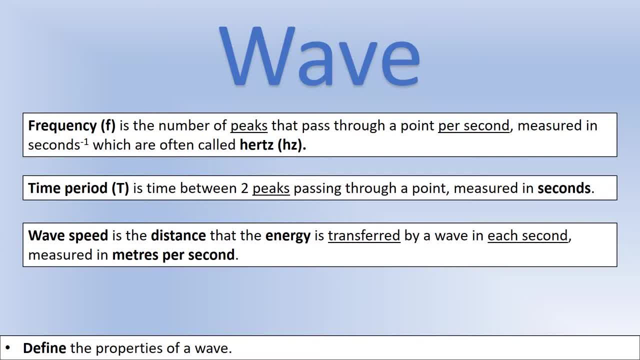 named after a famous scientist called hertz um, but it has a base unit, or a fundamental unit of seconds minus one or one over seconds. that's what a hertz is. the next is the time period, which is the time taken between two peaks passing through a point. so essentially, what that means is: you're if you're. 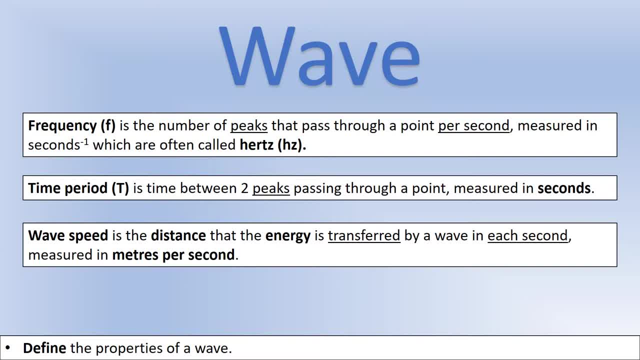 trying to visualize this. you are sitting at a point and you just count the number of waves that go through that point in a second. that would be the frequency if you measured the time between the two peaks. that would be the time period and we'll look at the relationship between. 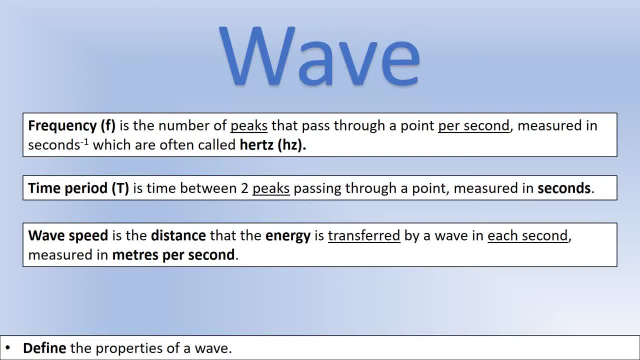 those two a little bit later on. and the final thing we might be interested in waves is the speed, which tells us the distance that energy is transferred each second by the wave. that's what we really mean by wave speed. we're measuring how fast the energy moves, okay. 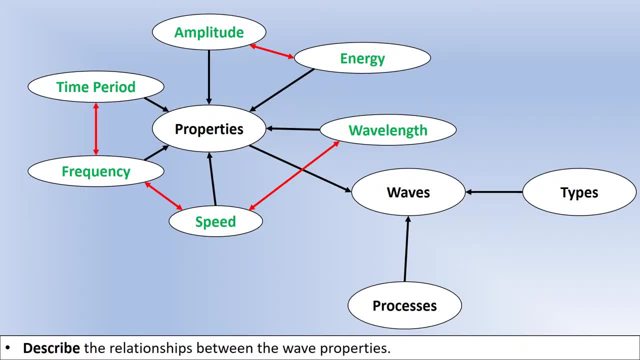 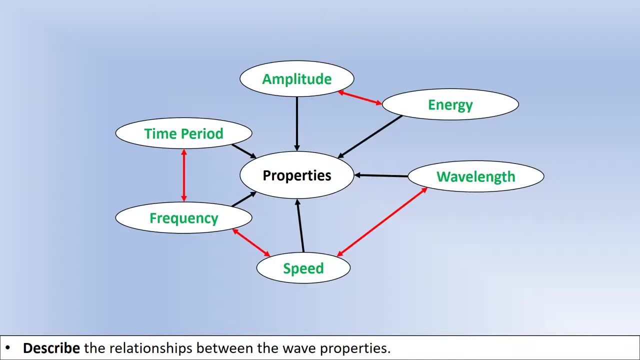 are our properties of a wave. now, as you can see from the red lines, we're going to explore the relationship between these different properties, and so i already mentioned properties that are linked together. let's now explore what the specific relationship is. so these are all things that have been determined experimentally and you figure out these. 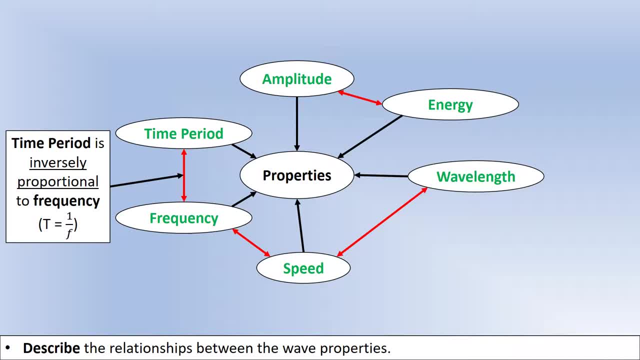 relationships. so the first one we're going to link is time period and frequency. so what you find is that time period is inversely proportional to frequency and the, the constant of proportionality, is one in this particular relationship. so we get this equation: time period is equal to one over frequency, or the reciprocal of frequency as it's sometimes called. 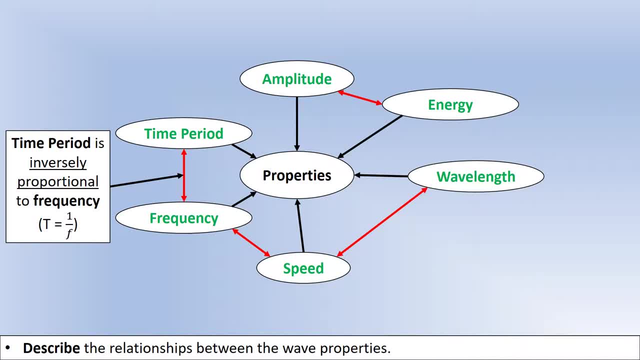 so that's a nice simple relationship between those two, and what that means is, if you measure time period, you now know what the frequency is, or if you measure frequency, you know what the time period is straight away, which is quite helpful. the next one is the relationship between amplitude and 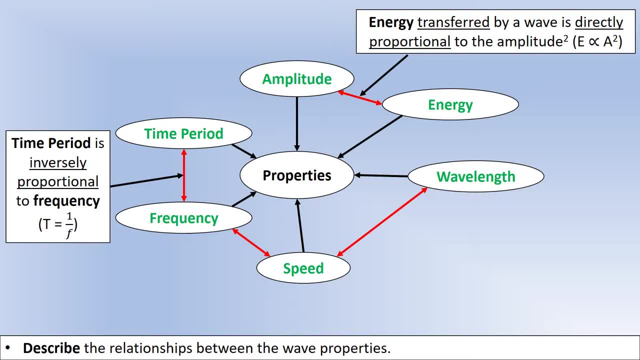 energy, which i mentioned earlier. so the energy transferred by wave is directly proportional to the amplitude squared. and what the friend is? you gonna look upon this as it takes date over day and now, as a lot of you, can do anything, and then you, Karina, will get to닥term jeunes and find some. 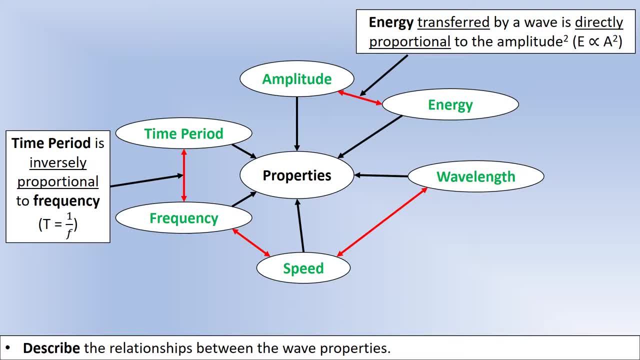 ibi to help you out a little bit more and then a lot. the other problem we're actually going to look up is if theivos are. So what that really means is if we double the amplitude, the energy transferred will be multiplied by four, because it's proportional to the amplitude squared. 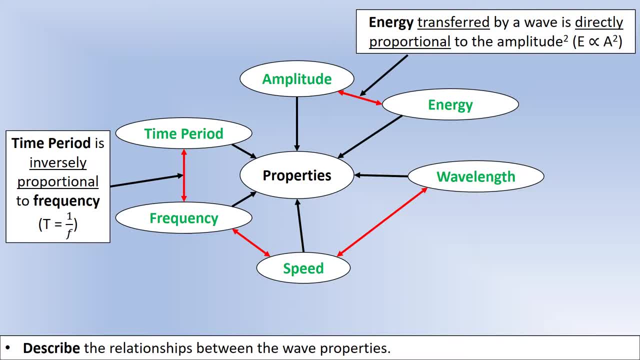 So that's why I said it's a measure of the amount of energy being transferred. And the final equation is a way of linking frequency, wavelength and the speed at which energy is transferred, And we have what's called the wave equation. So speed is equal to frequency times by the wavelength. 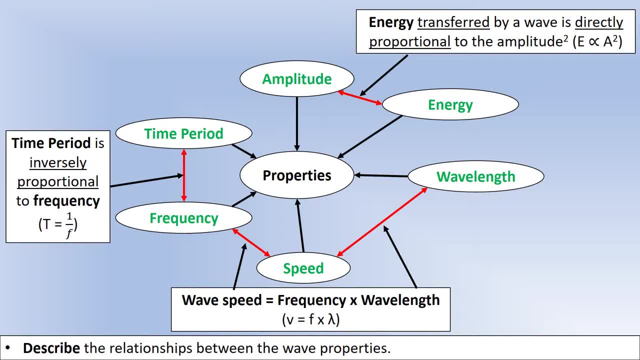 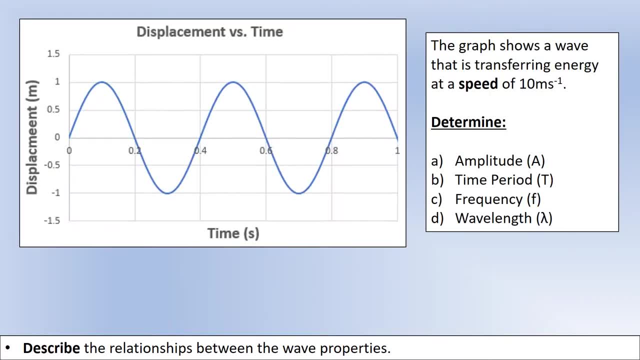 So that relates the last three properties of wave. OK, so those are the relationships. Let's put these to use. So I'm going to ask you a series of questions And what you're going to do is you take some either measurements from the graph or use the equations that we I've just shown you to try and work out some different properties of the wave I'm showing you. 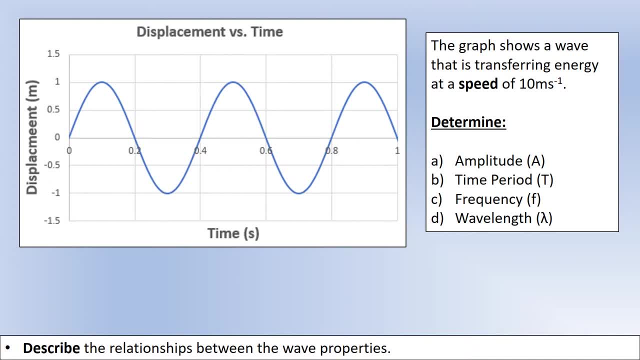 So we've got a displacement versus time graph Here And it tells us we've got a. the energy is being transferred at a speed of 10 meters per second. So what I'd like you to do is pause the video now and see if you can work out each of these properties. 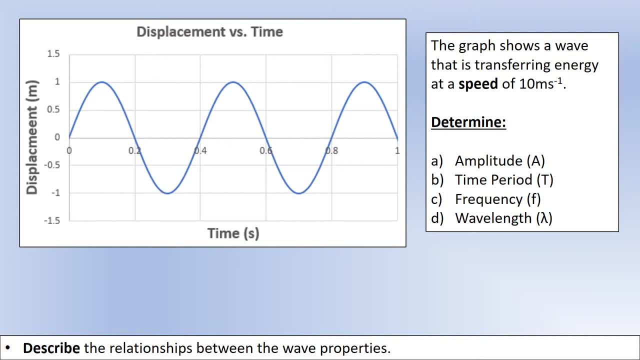 So the first few, you'll just be able to measure off the wave. The last couple, you're going to need to get the equations out to do some calculations with. So pause the video now and have a crack at these questions. OK, so now you've had a chance to have a go, and it's really important. 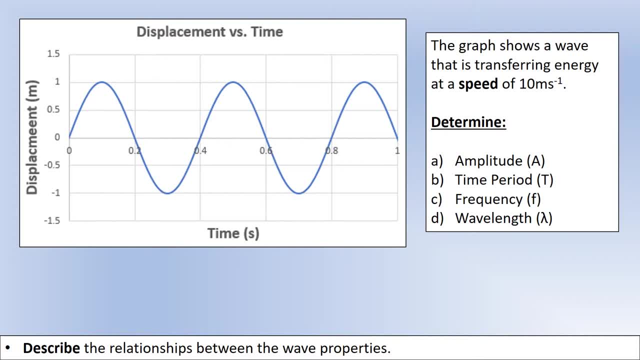 That you've had a crack at each of them. Let's take a look at what we should have. OK, so the first two, as I said are, can be measured from the wave, and there are a few different points. you can measure them. 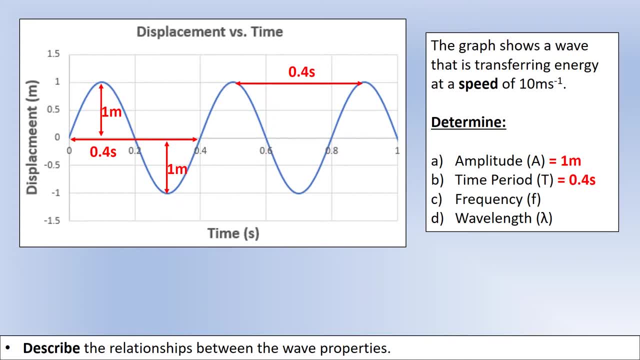 So first, amplitude we would measure from the center line And if we measure it to either the peak or to a trough, we can see that we get as one meter Because we've got a displacement versus time graph. that means the distance between the same point. 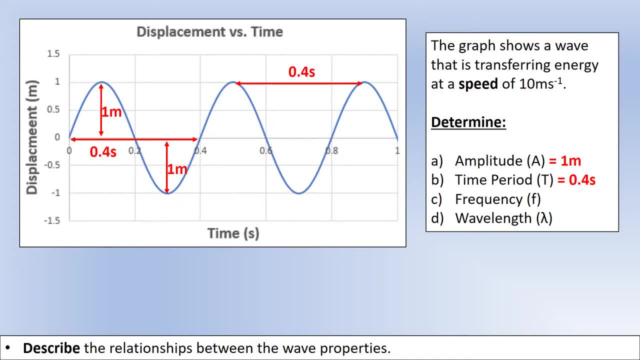 And the wave would be the time period for this particular wave. So there are two particular points I think would make sense to measure it from. So both of them give you a time period of not point four seconds. So either of them would be fine. So those are the two straightforward ones to measure from your wave. 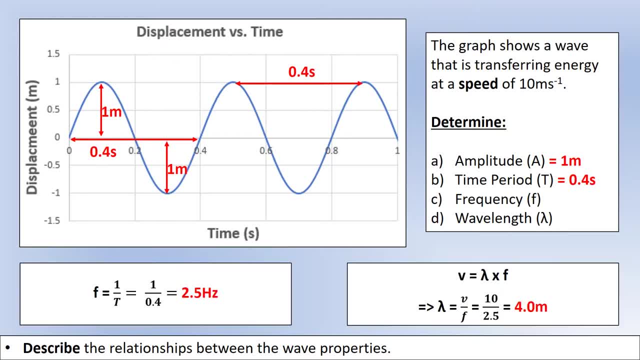 Let's now look at the ones we're going to need to do some calculations for. So, first off, we can calculate the frequency- Now we know the time period- by just doing one divided by the time period. That gives us a frequency of two point five hertz, which you can see at the bottom left. 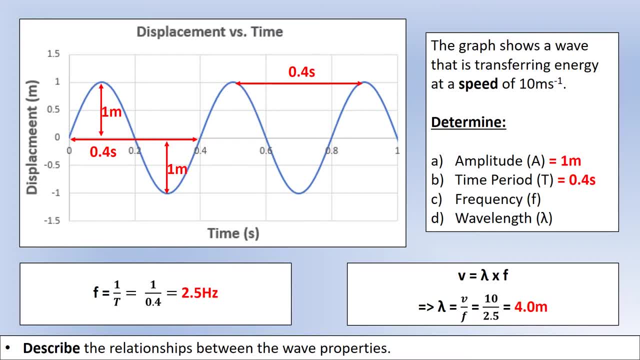 And then to get the wavelength, we're going to need to use the wave equation. So the first thing we're going to do is make the wavelength the subject of the equation by dividing both sides by frequency, And then we've been given the speed is 10 meters per second. 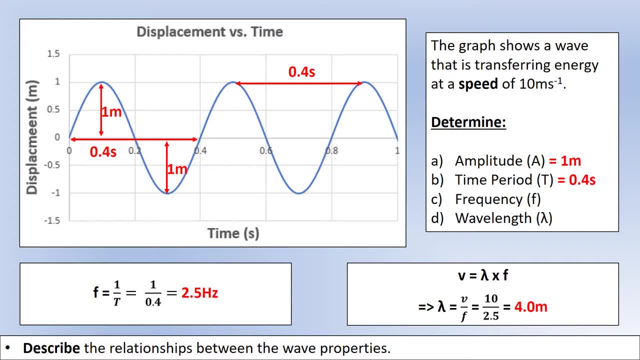 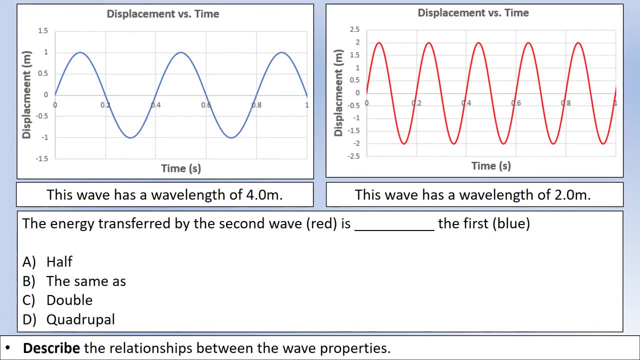 We've got. the frequency is two point five, So that gives us a wavelength of four meters. OK, so that's doing some basic calculations Of properties of wave. Let's now have a look at comparing two different waves using the properties. So the first thing we want to do is compare the energy transferred by the red wave to the first wave. 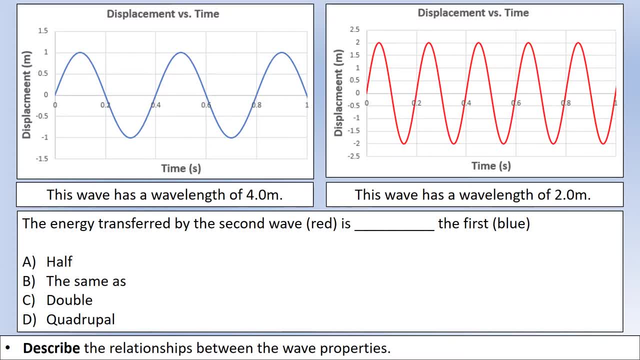 So what I want to do is pause the video, have a look at, maybe taking some measurements from these waves, and see if you can come up with the relationship between the red wave and the blue wave. So, for instance, maybe you think the red wave has double the energy. 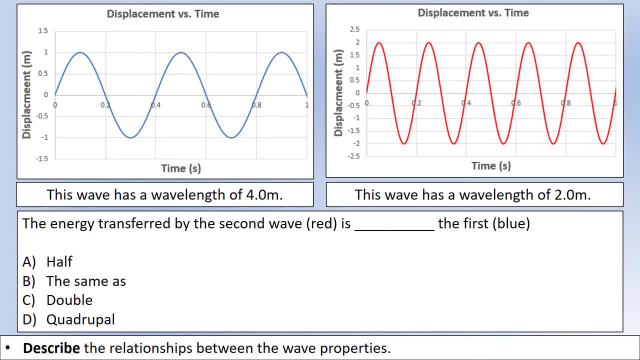 Well, half the energy, or the same energy, transferred. So pause it and have a go, and then we'll review it. OK, so now you've had a chance to have a crack The. the key thing here is the amplitude. So you can see, the red wave has double the amplitude of the blue wave. 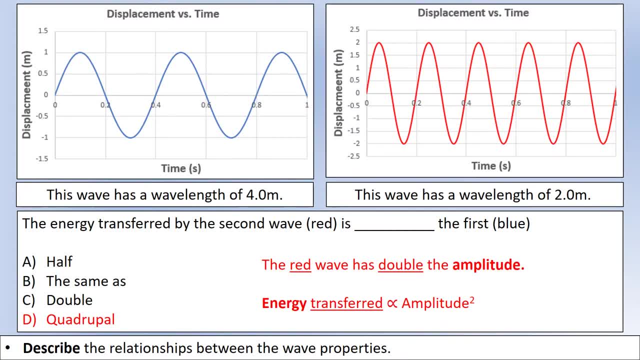 So what a lot of people do would now would incorrectly select that and say that the energy transfer is double, because they forget that the energy transferred is diaporting to the amplitude squared. So what that means is, if you double the amplitude, that means you're going to transfer for four times as much energy, which is why we would pick quadruple the amount of energy for this particular one here. 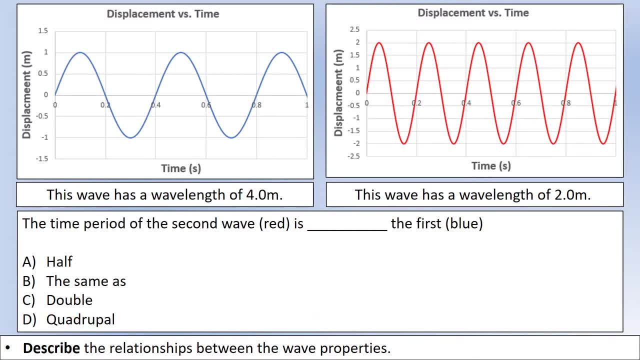 OK, so same two waves. We're now going to compare them in terms of their time period. So again, pause the video, select your answer, then we'll review it as before. OK, so let's take a look. So from the diagram we can measure the red wave. 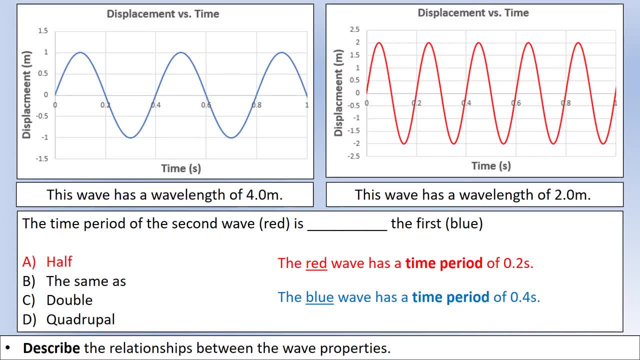 The red wave has a time period of not point two seconds. The blue wave has a time period of not point four seconds. This is the same wave that we were looking at before, So therefore the red wave has half the time period of the blue wave. 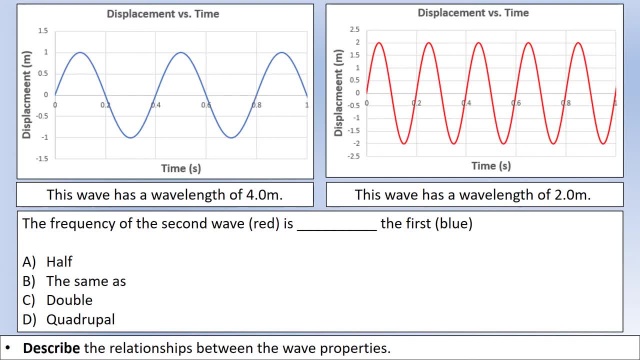 OK, so let's now compare the frequency. So again, pause the video and have a crack at this. These are the same two waves, So you might be able to calculate it, but there are a few ways of doing it. See if you can figure out the relationship. 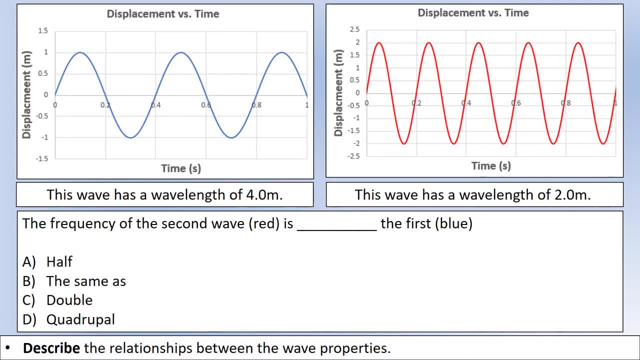 So we're going to be using the red wave and blue wave for frequency, All right. So if we have a look at the red wave, we can see that in one second we've had five complete wave cycles. therefore has a frequency of five hertz. 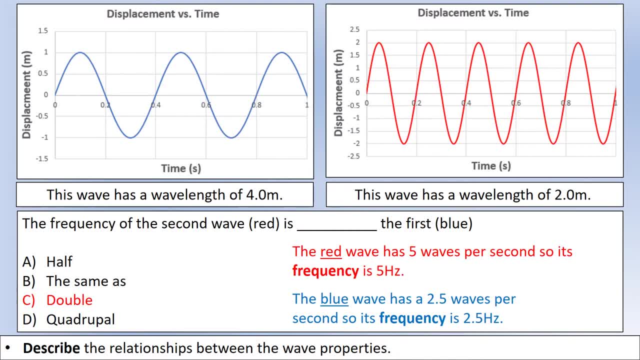 The other way we could have done. that is, we know the time period of the one on the right is not point to one divided by not point two is five hertz as well. So there are two ways of doing that. Blue wave We can see. 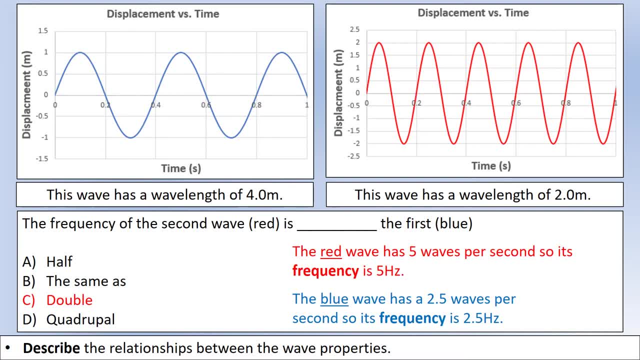 We can see that the red wave has two point five full cycles during one second. So that tells us two point five hertz. We also calculated its frequency earlier as two point five. So we can see they're the same. So we see the red has double the frequency which we, which makes sense because it had half the time period. 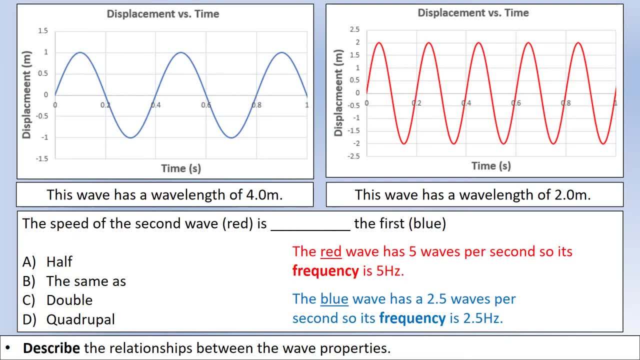 So that makes sense too. OK, so let's now compare the speed of the two waves So you can see. we've been given what their wavelength is: four meters and two meters. So I'd like you to have a crack at this. 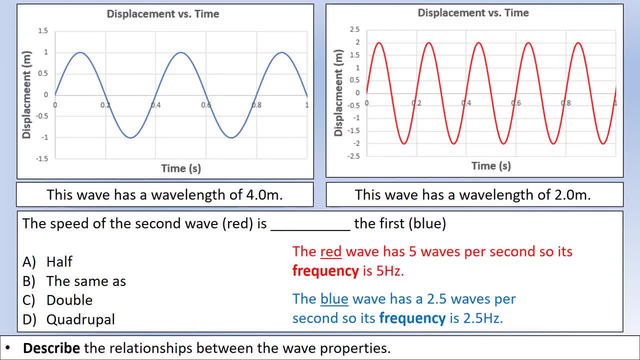 And I've given you the frequencies we've just calculated there. OK, so now you had a chance to pause and have crack. Let's have a look at this one too. So the red wave has a frequency of five hertz, a wavelength of two. 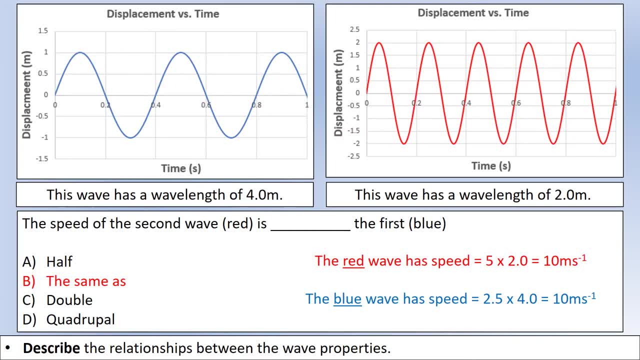 So five times two gives you a speed of 10 meters per second. Blue wave had a frequency of two point five has a wavelength of four. Therefore its speed is also 10 meters per second. So the correct answer you should have got here is that they should have been the same as each other when we've calculated them.